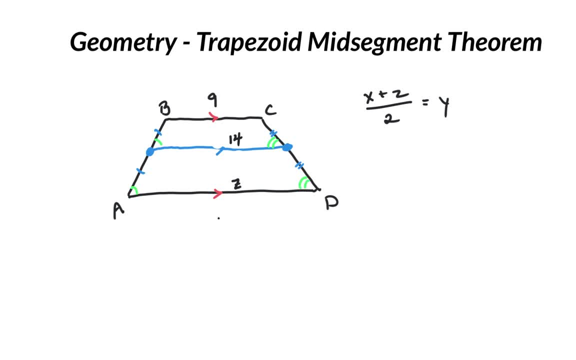 Well, using our same formula. we don't know what z is, but 9 plus z, divided by 2 equals 14.. Well, we could multiply both sides by 2 so that that divides out. So then, 9 plus z, divided by 2, equals 14.. 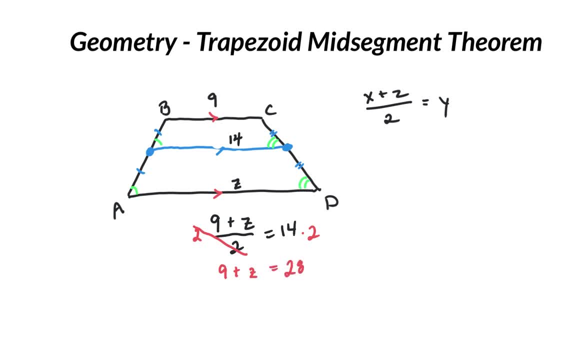 So then 9 plus z, divided by 2, equals 14.. So then 9 plus z equals 28.. We can subtract 9 from both sides and we get that z is 19.. Now, another way to think about this is that when you do an average of just two numbers like this: 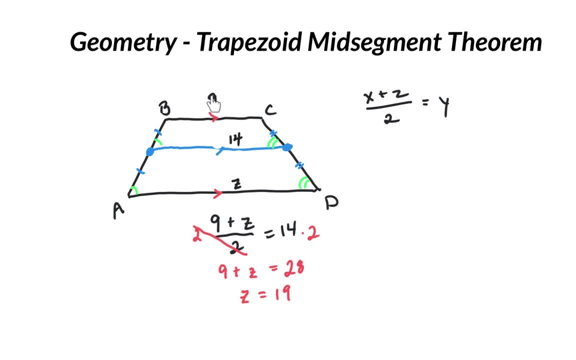 if the difference here was 5, you know, we went: our small base was 9 and plus 5 was 14.. Well, plus another 5 would give us the other one. So that's another way to do it, The opposite. we could also go the other way. 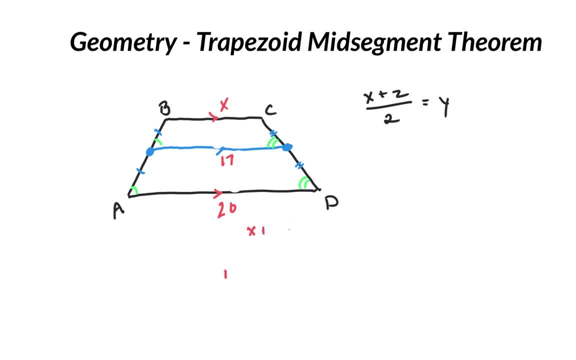 You know we could say all right, x plus 20 divided by 2 equals 17,. multiply both sides by 2, so we've got x plus 20 equals 34, subtract 20, so x is 14.. 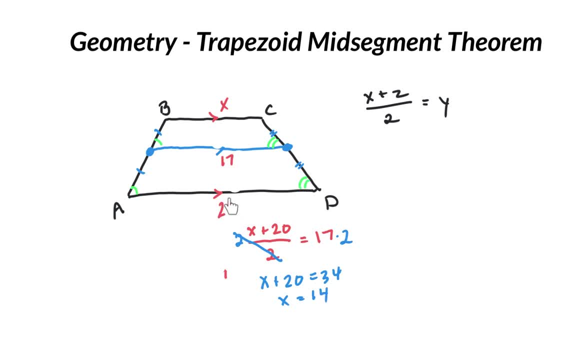 But again, if instead you said, well, this was 20 and this was 3 units smaller, 3 units smaller again would be that 14.. So again there's some algebra we can do here and some good problems we can do with the triangle mid-segment theorem, excuse me, trapezoid mid-segment theorem.